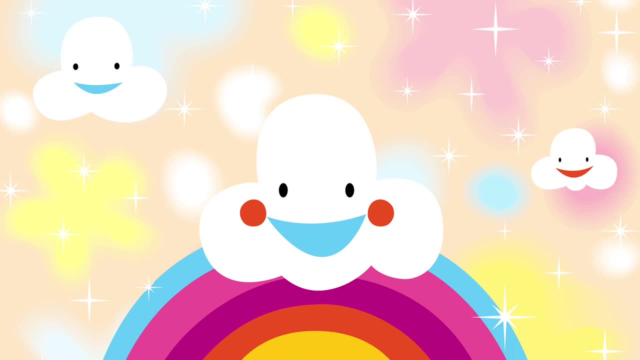 in your lap. Decide now which works best for you and get settled. Now. let your body be still. Your eyes are open so you can blink, but they're not looking at anything in particular, Just softly looking ahead. Can you feel your breath moving, Coming in through your nose and then out of your mouth? 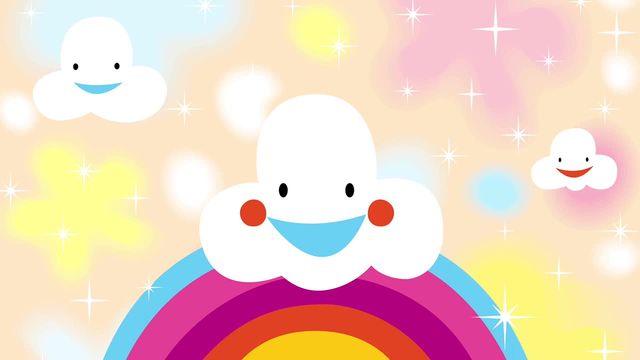 See if you can just watch it Coming in through your nose and out of your mouth. That's it Good. And one more With this one. as you breathe out, just let your eyelids softly close. Well done, Now all you have to do is listen to my words and enjoy the pictures that appear in your 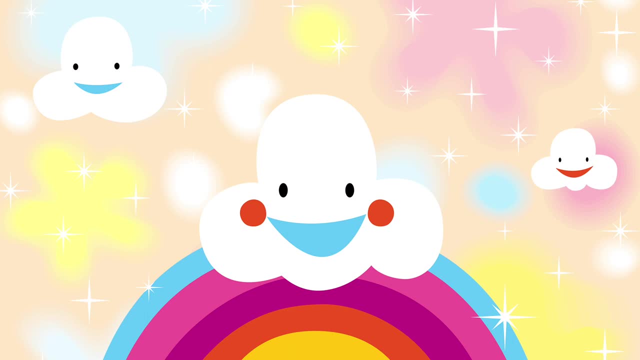 mind. If the pictures aren't happening, it means you're not listening. It probably means you need to relax just a tiny bit more. so breathe deeply and sink your body down further, Be peaceful and simply listen. Imagine you lying on your back on the softest green grass. I don't feel a thing, growing and leaving me all clean and all feeling great. You're still trying to find a way to be as just as comfortable as possible, making more of a difference to yourself and building your relationship with theелен's life. Mind your vision. Instead of remembering the world, think about all of the things hitherto close to you all apologize for, and forget about your collarbone or all of those you want to do The rest of the day. you safely set, if you can, and it slowly start working. 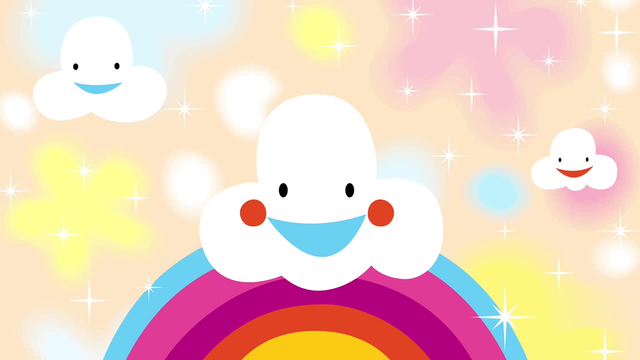 grass in a garden or a place you know, a park maybe, or just a big wide open field. As you lay here, you see the huge blue sky above you. In the sky you see lots of fluffy, puffy white clouds. 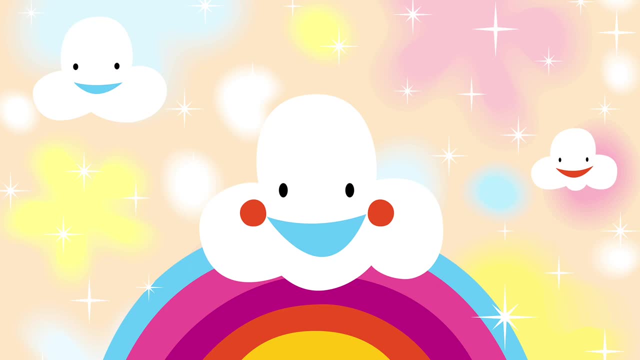 As you look at the sky, you notice that the clouds are making shapes, Shapes of things that you recognise. There's one, the shape of a rabbit: You can see its ears And the shape of its nose. Another is the shape of a whale, with a huge body and a fork-shaped tail. 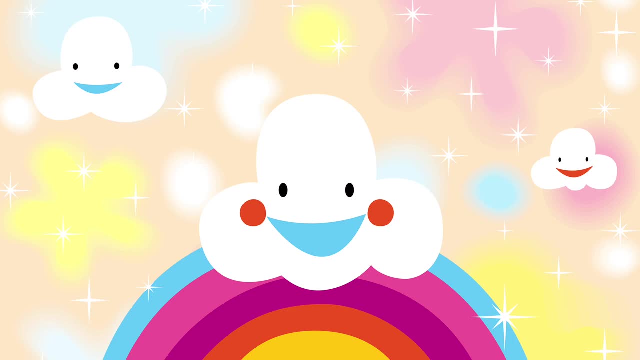 Oh, look a crocodile-shaped cloud And it looks like it's smiling. That one looks like the letter C A- ginormous pear. And it looks like it's smiling. That one looks like the letter C A- ginormous pear. 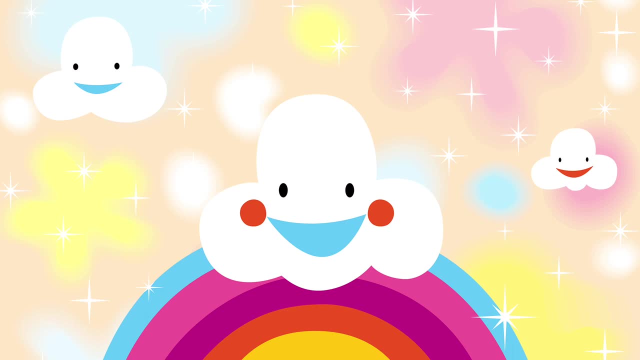 And it looks like it's smiling. And it looks like it's smiling. A puffy letter C And that one looks like a house. It has windows, A bubbly-shaped roof And a chimney, With a wispy bit of cloud making a twist of smoke. 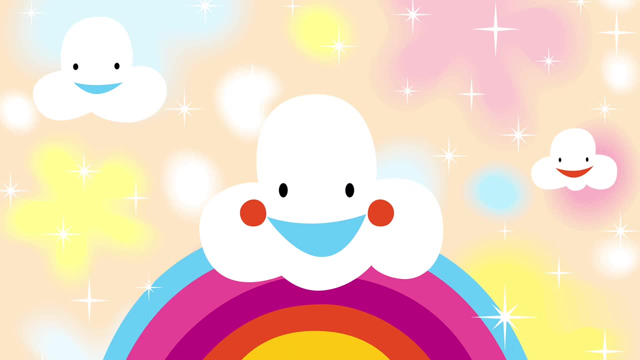 Maybe a cloud-shaped person lives inside. As the clouds move across the sky, the shapes change, New ones appear. It's like the sky is telling you a story. by painting pictures with the clouds, You see the shapes and you can put them together to make a story. 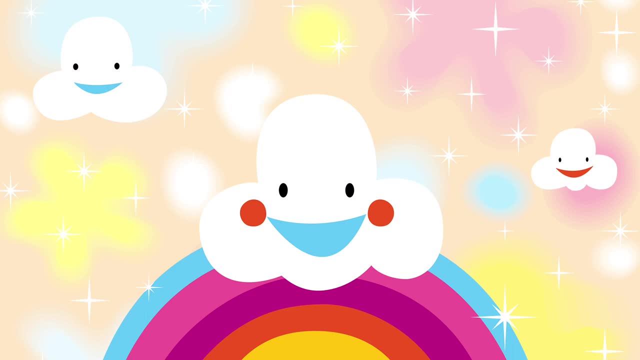 What other cloud shapes can you see, Watch, Enjoy them. You decide what the shapes remind you of. It feels great to know that you can make cloud shapes here in your mind And you can see them in real life too. Cloud watching will always help you feel calm, free and thankful that you are here in this beautiful world. 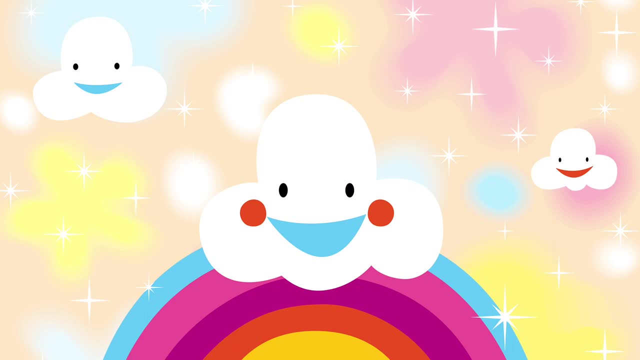 There is so much that is beautiful, Even everyday things like clouds that are there all the time. It's time to come back into the space around you, Back into your body again. Start by noticing how your body feels, here on the floor or the chair beneath you. 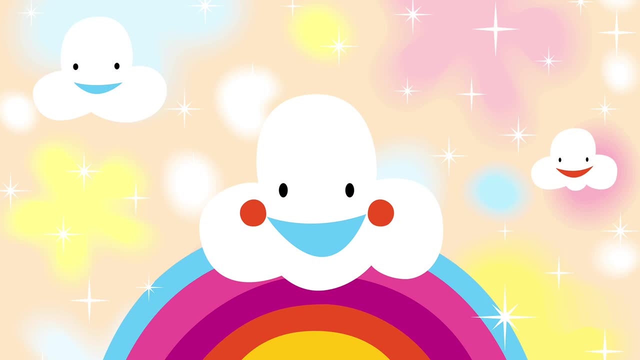 How heavy it feels. Now listen and see if you can hear any sounds around you- Ones nearby And others far away. Now take a big, deep breath in through your nose And sigh out from your mouth. Have a little stretch, Move a little. 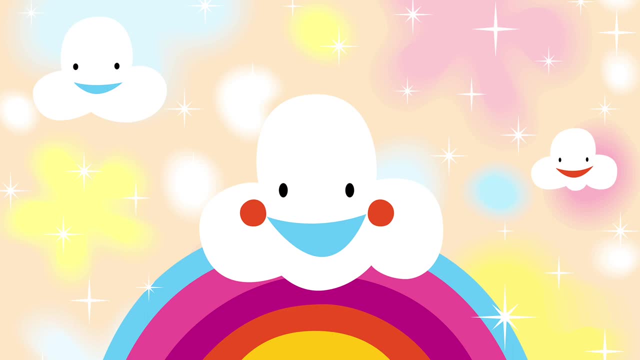 Jiggle your fingers, toes, ankles and wrists And gently open your eyes Just for a moment. sit back And notice how you feel after that. Do you feel different to how you did before? Well done for taking a few moments to look after yourself. 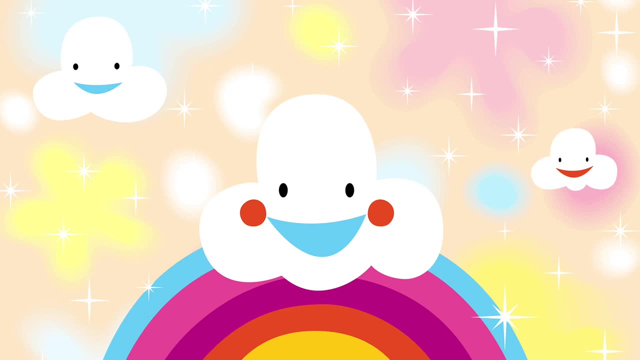 And now take a deep breath in Your mind and body will now be all the stronger for it. And remember the sky is always there to remind us to be open to ideas, To believe that anything is possible. I hope you try cloud watching outside in real life one day too. 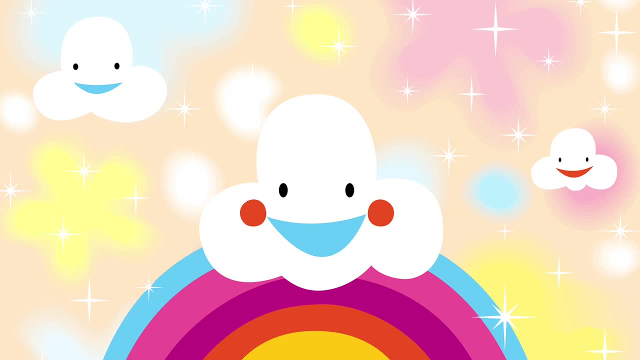 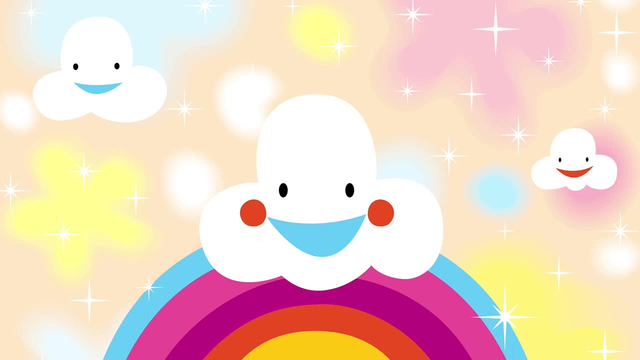 Maybe, Maybe, Maybe, Maybe, Or write it down, if you like. Your story will be different to everyone else, As only you know what the shapes look like. You are free to make them into whatever you like. I'll see you again soon. 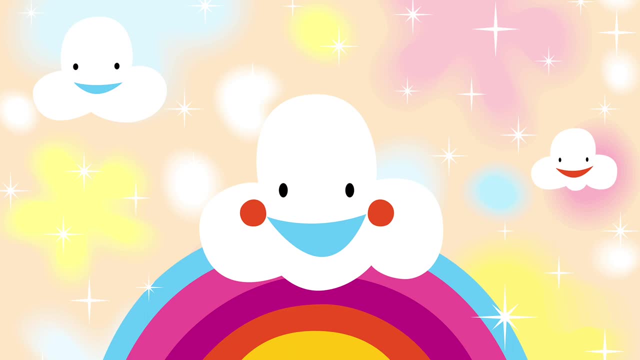 This is Jamie saying peace out.